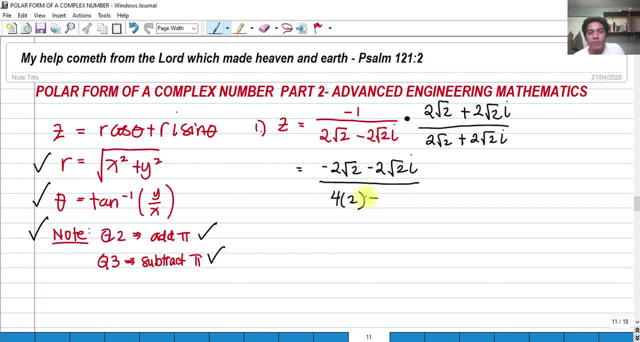 that should be two. Okay, negative times positive, that would be minus. we have two times two, that's four. squared of two times squared of two is two And i times i is negative. I squared, which is again I squared, is equal to negative 1. so we have an answer. 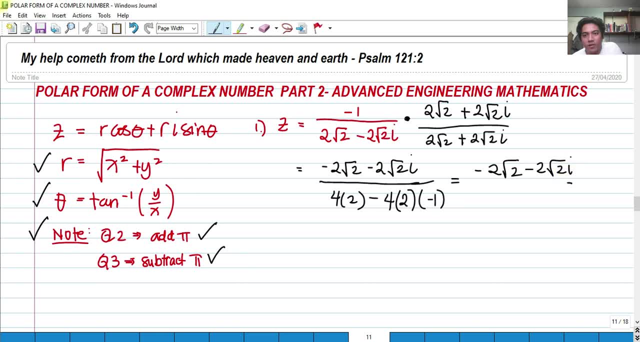 negative square root of 2 minus 2 square root of 2i over 8: okay, and this would be negative times negative would be positive. so 8 plus 8: okay. so we have negative 2 square root of 2 minus 2 square root of 2i all over 16 and we can. 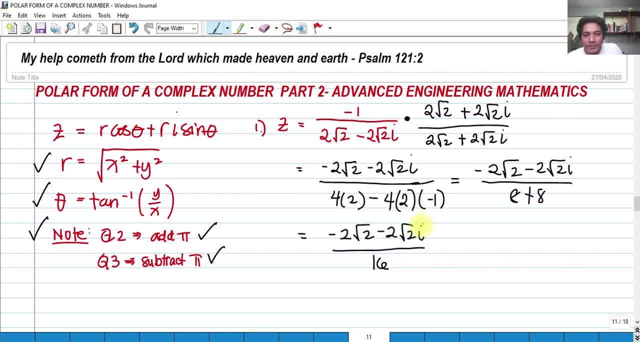 simplify this. we can simplify this as negative: 2 square root of 2 over 16, minus 2 square root of 2i over 16, and we know that this can be cancelled. so we have 8 here, okay, so what will happen here? we simplify this as negative square root of 2. 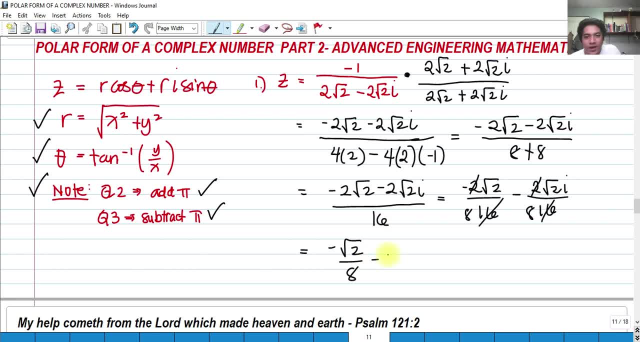 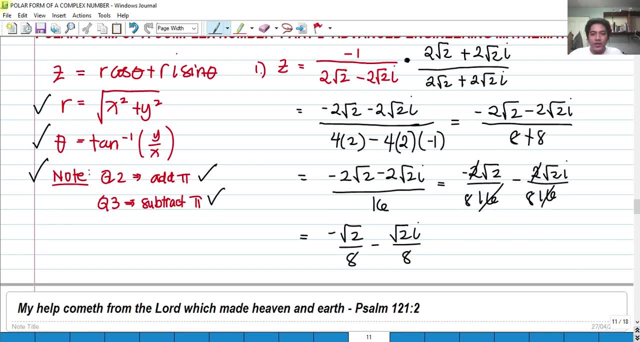 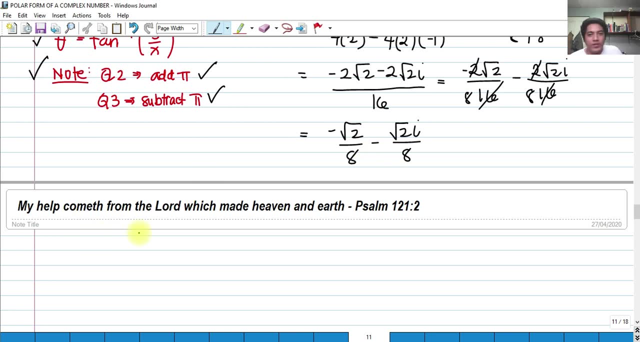 over 8, minus, okay, square root of 2i over 8. so, anyway, now we can actually convert this into polar form, because it is actually in a simplified form, so we can get r as negative square root of 2 over 8, squared okay, plus negative square root of 2 over 8. 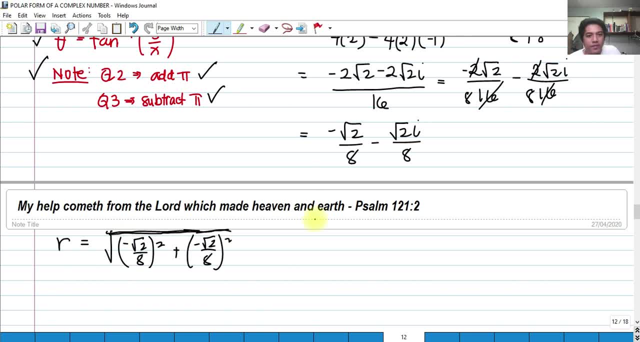 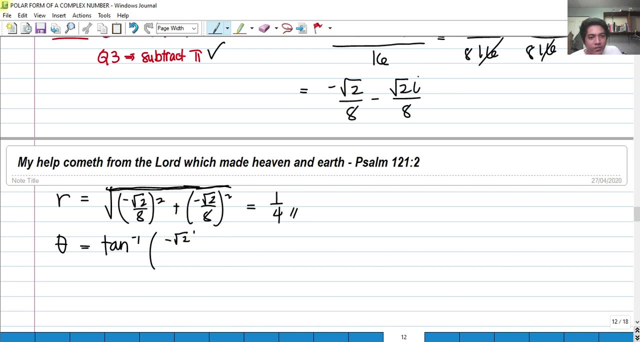 squared. that's a square root here, so our answer is 1, fourth, if you're going to calculate it. so our angle arctan is simply equal to 1, because this: these are the same. so we have negative square root of 2 over 8 divided by negative square. 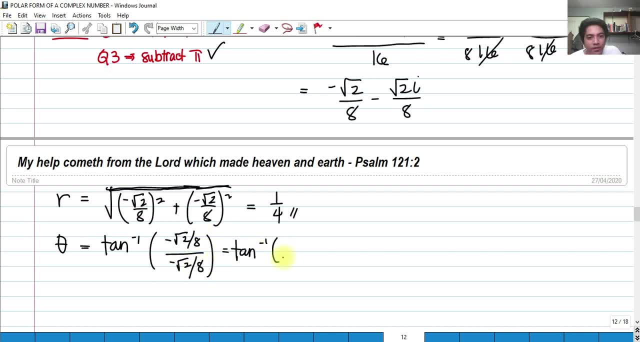 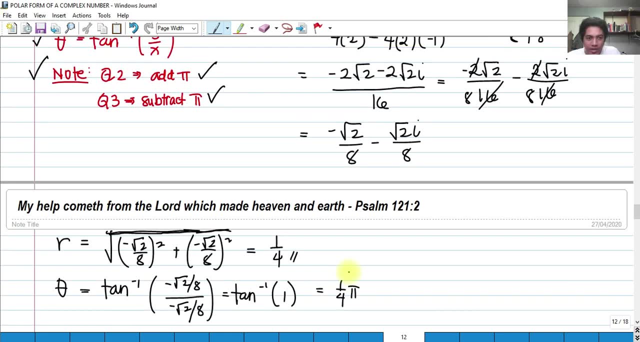 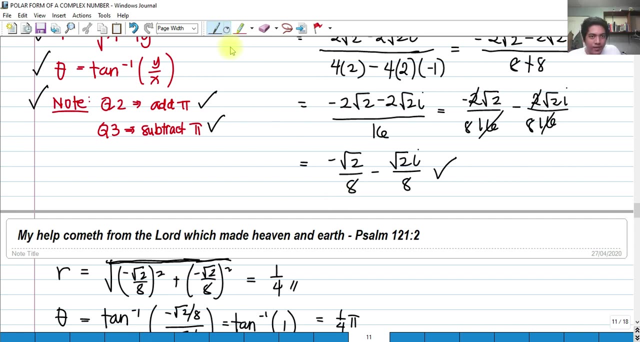 root of 2 over 8. that is simply equal to arctan of 1. okay, which is equal to 1. fourth, or pi over 4. again, take note that this complex number is located in the square root of 2, because 4 is a refusal. now, what we can do here is this: we quote: 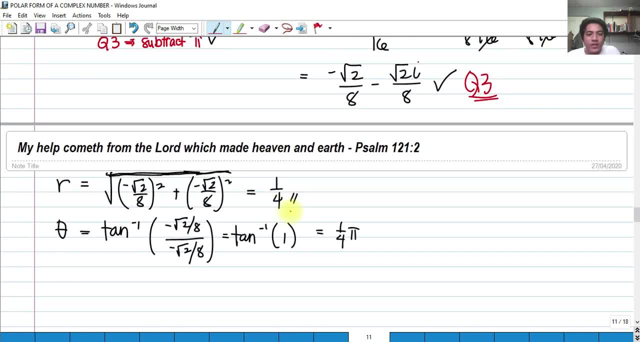 it can be shortly. form dictionary for bogusют. it can be spoken as a Mhm. they do not create selectively. we don't우�ريёмu populate n même than certificate thsthe expression we or not, because it is nwc. I was right, dangif». 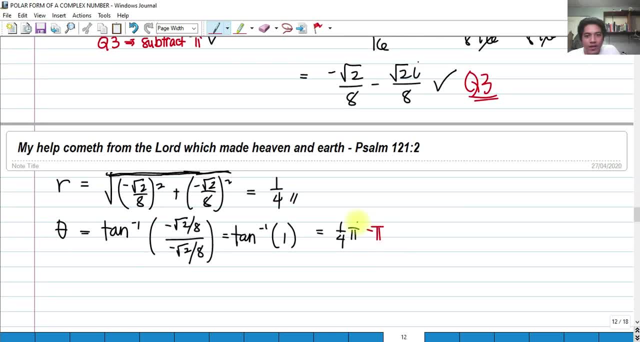 so Would that be 3 negative? we have a negative here and the negative here that's fot trees. that's to draw three. okay, not this in quadrant 3. so what are we going to do here? is this quadrant tree? we have to subtract pi from what we get on our 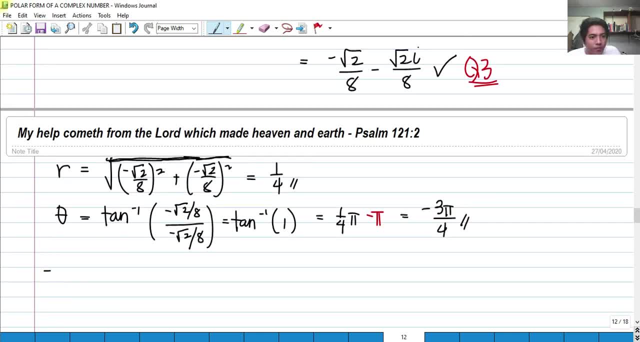 calculators. so let me first check what's happening. if you subtract by, that is negative 3pi over forth. so it means that the polar form of negativeizo, who ever Square root of 2 over 8 minus square root of 2i over 8, is now equal to what? 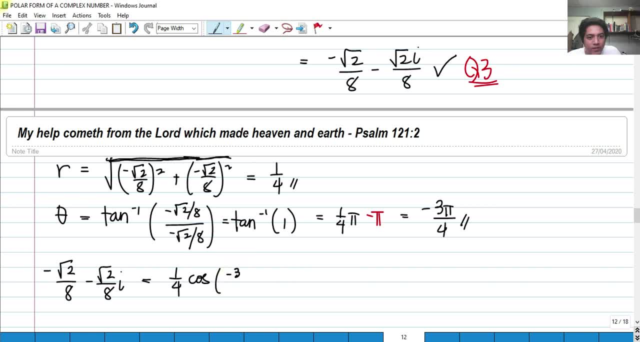 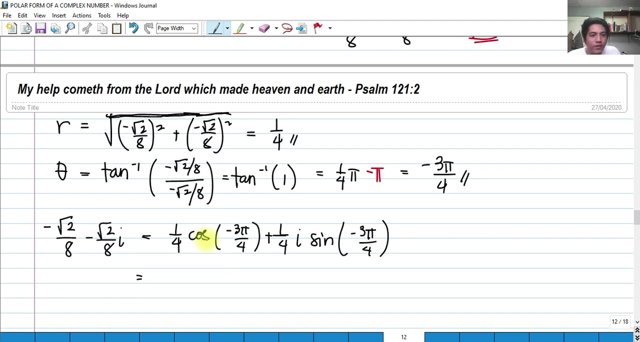 To 1 fourth cosine of negative 3 pi over 4 plus i sine of. I'm sorry, that should be 1 fourth i sine of negative 3 pi over 4.. Or we can factor out 1 fourth so that it becomes cosine of negative 3 pi. 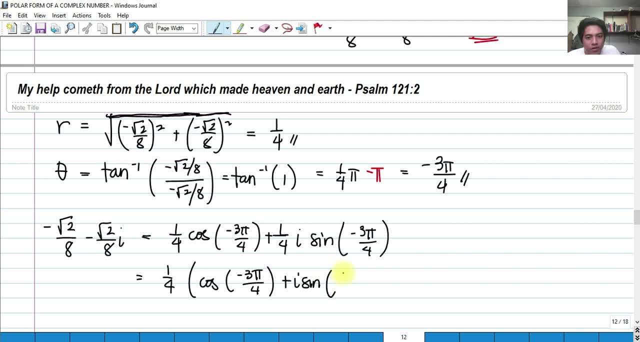 Pi over 4 plus i sine of negative, 3 pi over 4.. So, if you evaluate this, this should be equal to this. okay, So that's how we get the polar form for this problem. Okay, for number 2, let's try to solve this problem. 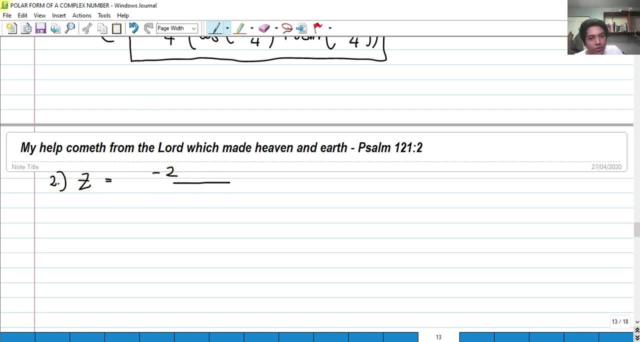 So we have: z is equal to negative 2 over 1.. Minus square root of 3i. Okay, so we need first to simplify this before we can apply our formula. So we can multiply this by the conjugate of the denominator. 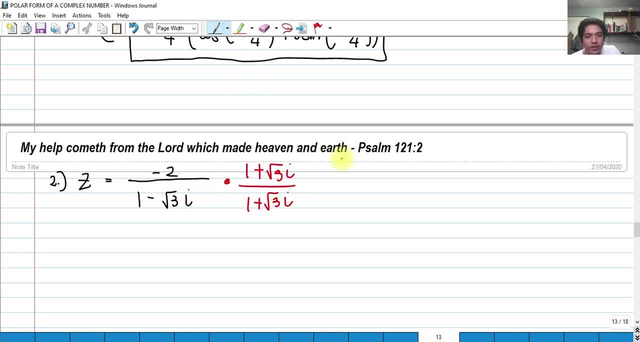 It's fine. Okay, we should simplify first this. So we have negative 2 minus 2 square root of 3i. for our numerator, For our denominator, we have 1.. Okay, we have 1 square root of 3 times square root of 3i. 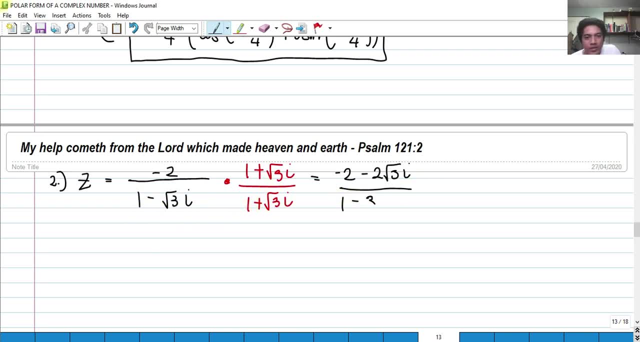 Okay, that's minus, that's 3.. i times ii squared, that is equal to negative 1.. So we have negative 2 minus 2. square root of 3i over, we have 1 plus 3. Negative 3 times negative: 1 would be positive. 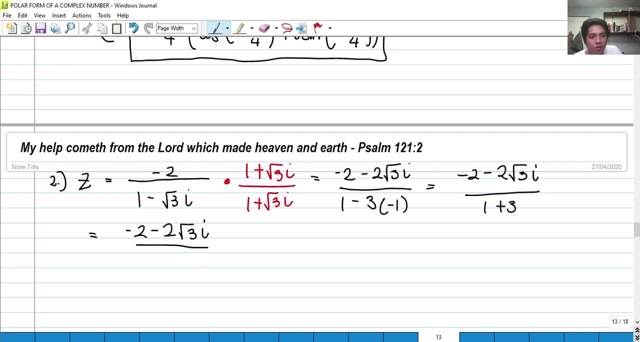 So we have negative 2 minus 2 square root of 3i all over 4.. We can rewrite this as negative 2 over 4 minus 2 square root of 3.. i over 4.. We can simplify this: Negative 2 over 4, negative 1 half. 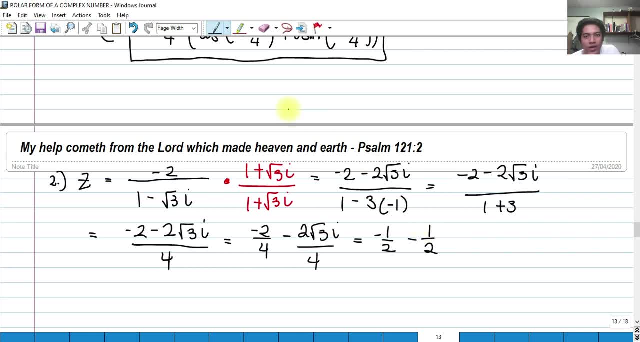 And this is negative 1 half also. Okay, or negative 1 half. This would this: would this 2 would be cancelled. Okay, so we have square root of 3i over 2.. Okay, so we have now this form. 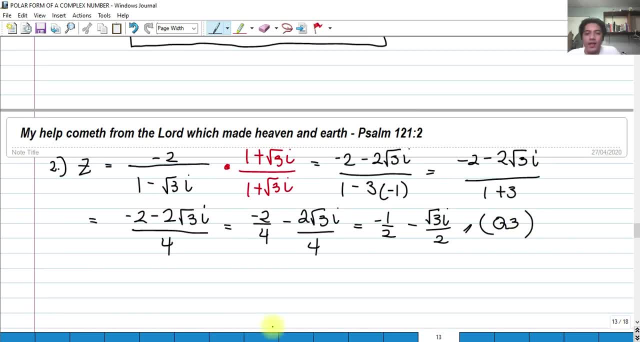 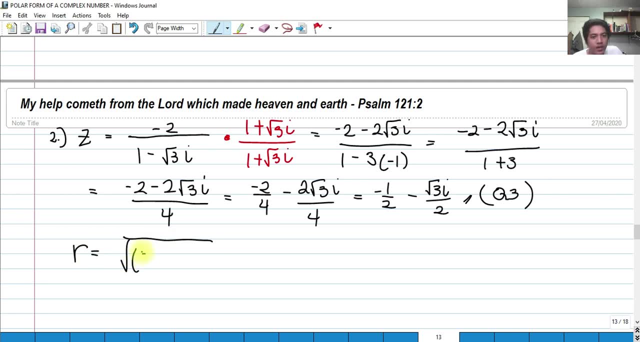 This is located in quadrant 3. So don't forget that if you get theta we should subtract pi. Okay, So if we get the r, r here in this case would be negative 1 half squared, plus we have negative square root of 3 over 2 squared. 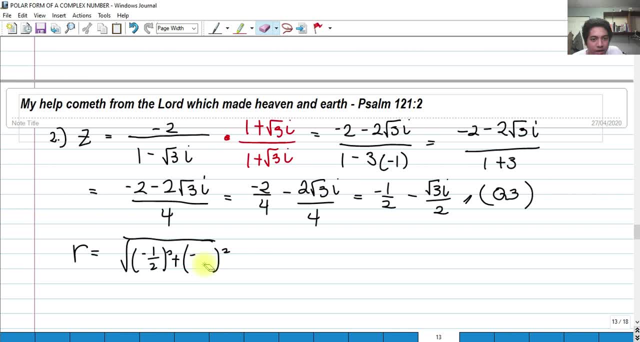 This is square root of 3.. Let me just rewrite this So negative: square root of 3 over 2.. So if we evaluate this, this is simply equal to 1.. Our theta would be: arc tan, Arc tan of negative. 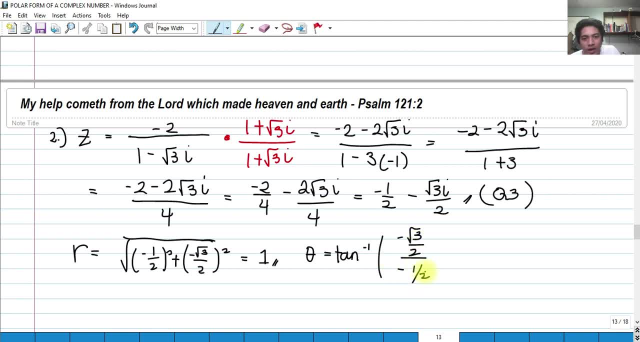 y, square root of 3 over 2 over negative 1, half, where 2s will cancel negative. square root of 3 over negative 1. that is simply the r? tan of negative or square root of 3. so whatever we get here, make sure that your calculator again is in radians, radian mode. okay, so we get what? 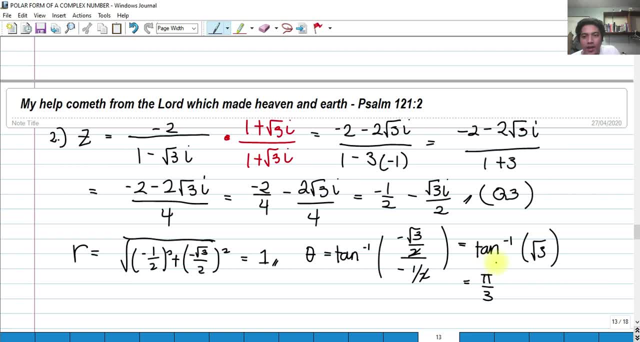 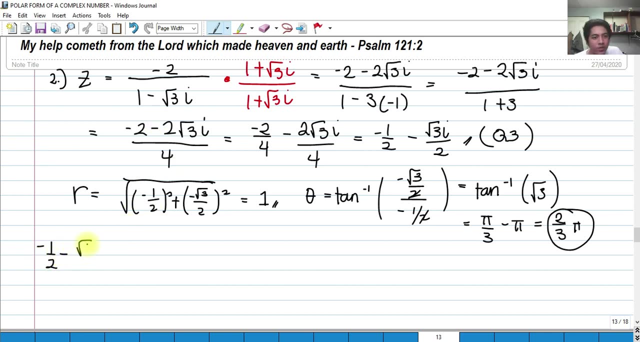 we get pi over 3 and since this is located in quadratic, we subtract pi, our answer for angle is 2 pi over 3. so our answer in converting negative 1, half minus square root of 3 over 2i into polar form is r cosine theta plus i r sine theta. so we have the value of r, which is 1. 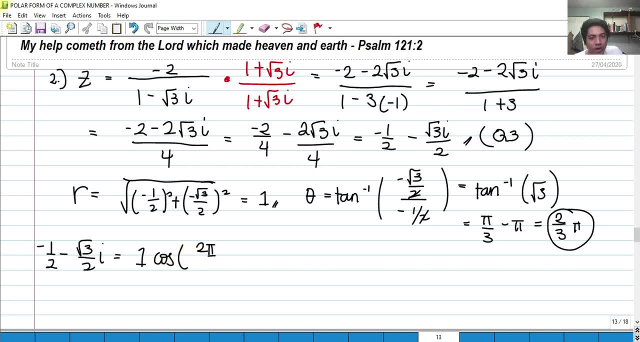 our cosine theta is 2 pi over 3 plus 1 i sine 2 pi over 3, or we can neglect putting 1 because it's understood. so this should be our answer. again, this is located in quadratic, so we have to subtract pi and. 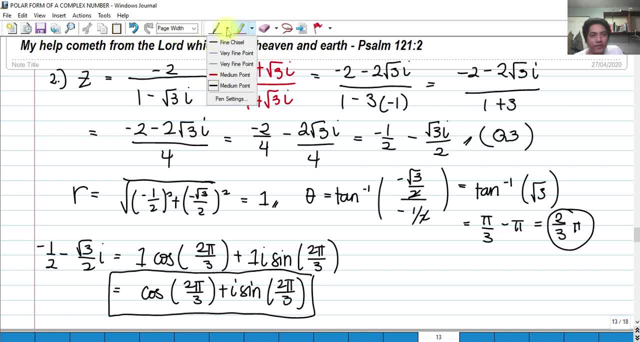 and uh, it is not positive: 2 pi over 3, but rather it's negative. it's negative: 2 pi over 3. okay, my mistake, that should be negative. so pi over 3 minus pi is equal to negative 2 pi over negative, 2 pi over 3. so this should be our. 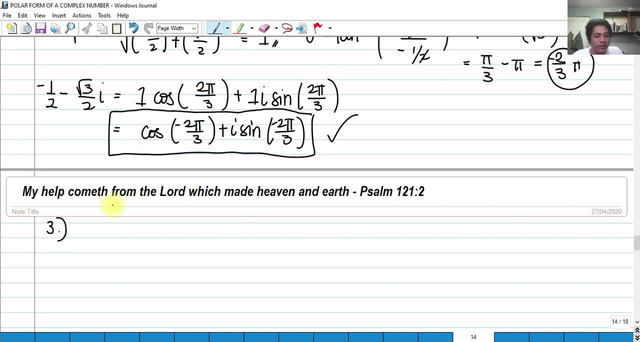 answer. so for number three, okay, the zay, the complex number is negative: 1 over 2 minus 2i. so it's До 2و Аy іلي reg 2O ll pri 4yl. 뭐야, the zay complex number is negative: 1 over 2 minus 2 i. so for the complex number is negative 1 over 2 i. 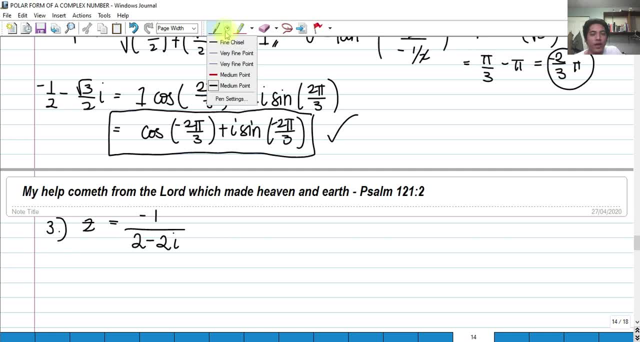 So minus 2 is going to beº 0 audience one negative. so it should always be negative: 2 pi over 3.. so how do again we can perform directly the substitution of r and theta here. so we have to reduce this complex number by multiplying by the conjugate of the denominator. so we have 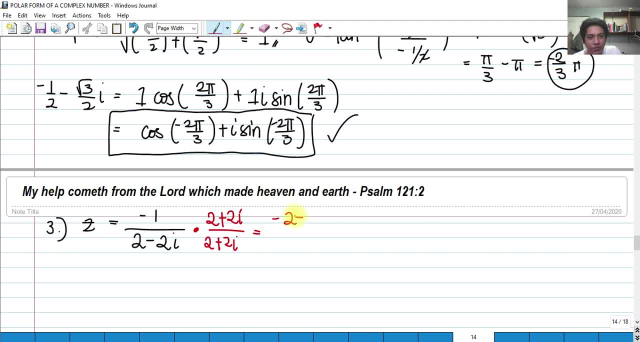 this, so it should be negative 2 minus 2i on the numerator. let me change my pen. it should be color black, so we have negative 2 minus 2i all over. we have 4 minus 4. okay, it's spoiled. okay. 4 minus 4 times negative 1 because i squared is negative 1, so we have 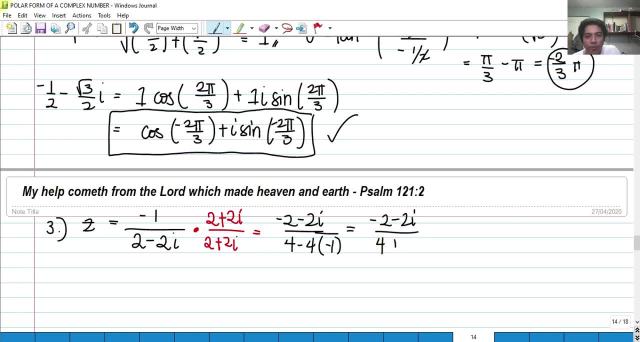 negative 2 minus 2i all over 4 plus 4, that is negative 2 minus 2i over 8, and we can simplify it by this. okay, we can rewrite it. so: negative 2 over 8 is negative 1 fourth minus 1 fourth of i. so this: 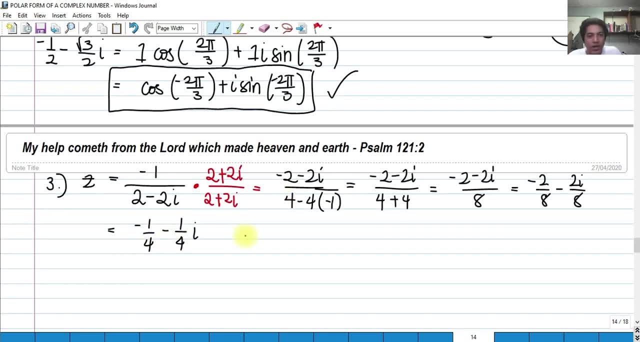 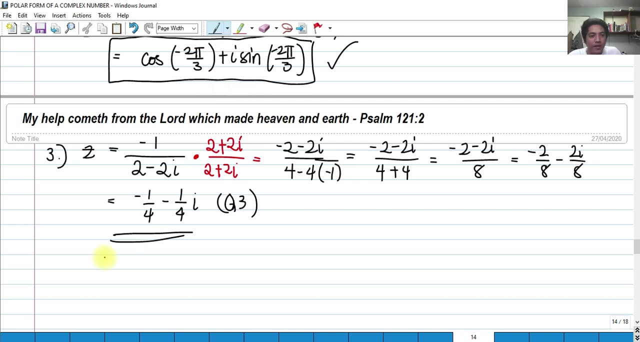 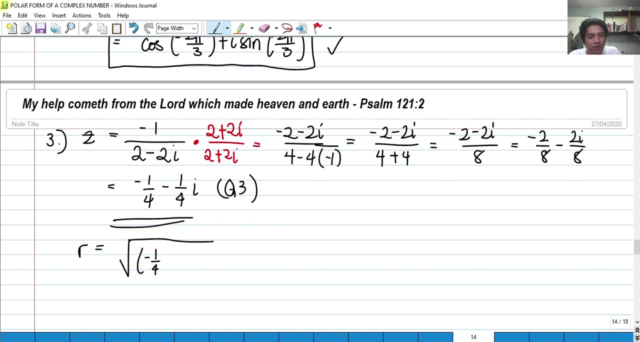 is our complex number, our simplified complex number. so again this is located at quadrant 3 because it is negative for our x and negative for our y. so we have to subtract pi again when we are getting the theta or the argument. so we have to get r. the r of that is negative 1 fourth squared, plus negative 1 over 4 squared. 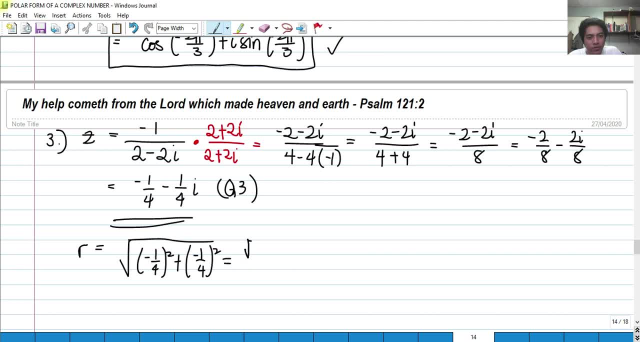 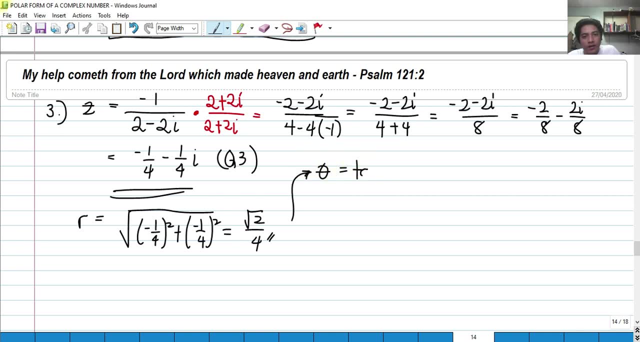 which in turns out to be square root of 2 over 4. that's our r for our theta. here, theta is arc tan. as you can see, that should be equal to 1, okay. arc tan of simply 1, okay. and the arc tan of 1 is pi over 4. so, again, this is what we get in our calculator. this is what. 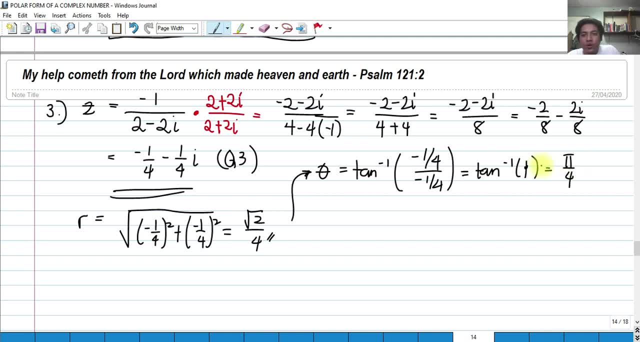 the calculator gave us. so we have to what? uh? subtract it from pi, because it's located in the quadrant 3, so we have theta pi over 4 minus pi. okay, so our answer would be negative: 3 over 4 pi. okay, that's our argument for the theta. 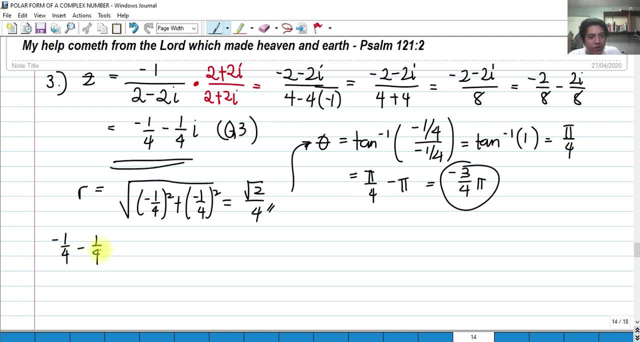 so negative 1, 4 minus 1, fourth i. in polar form, that is r, which is square root of 2 over 4, cosine of negative 3 pi over 4, plus square root of 2 over 4, i sine of negative 3 pi. 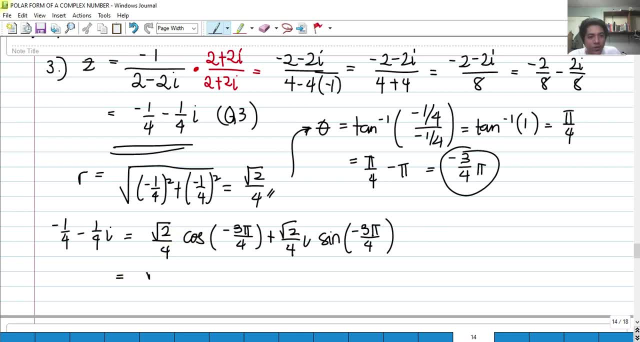 over 4 and we can factor out squared of 2 over 4, we have cosine of negative 3 pi over 4 plus i sine of negative 3 pi over 4. so this should be our answer for this problem. okay, for the next problem: the only way for you to actually get better in advanced engineering. 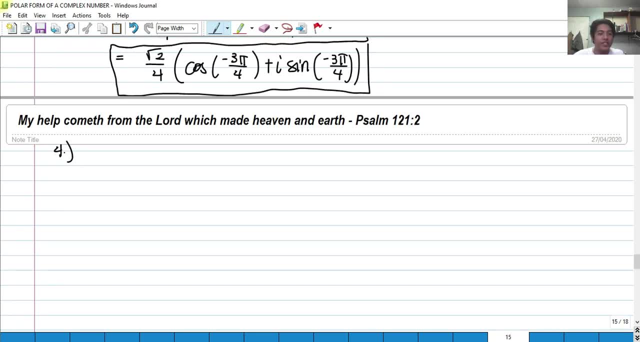 mathematics, and as well as in any other math subject, is to solve more problems, more problems, more chance of winning: 1 over 1 minus i plus 1 over 1 plus i. so we need to get the polar form of this uh complex number, given rectangular complex number. so, as we all know, we have to. 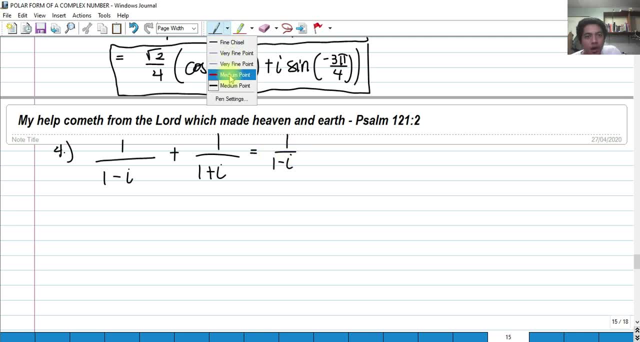 eliminate the uh i in the denominator by multiplying it by the conjugate okay, okay, okay, okay. so that's for the first term. and secondly, we have plus 1 over 1 plus i, so the conjugate of it is should be uh. they are not the same uh denominator, so we cannot easily uh multiply. 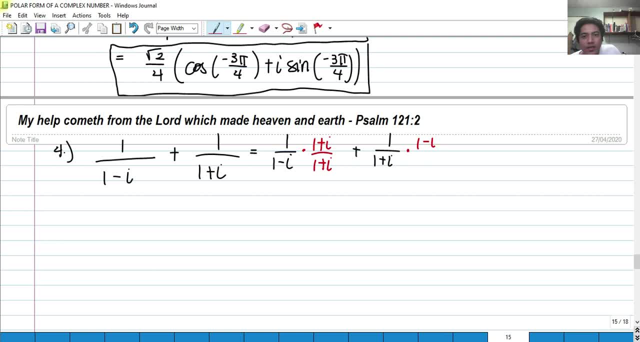 add them. okay, so we have to eliminate t i in the denominator. okay, so the conjugate is 1 minus i for this term. so we're going to perform it. what will happen is that this would be simply 1 plus i and this would be 1 minus i squared. i squared is negative 1. okay, and for the second term we have 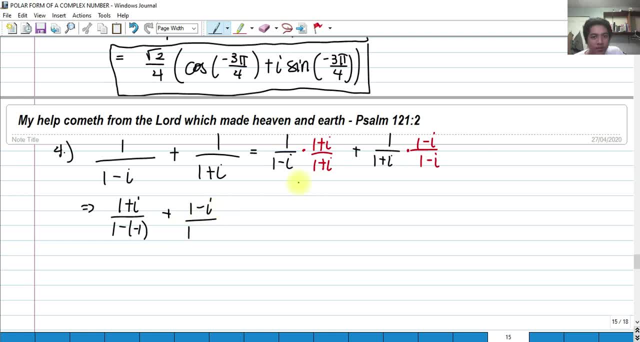 1 minus i. oh, this is 1 minus i squared is negative 1 also, so we have 1 plus i plus, 1 minus i over. this is 2, so we can actually combine them. this is 2: 1 minus negative 1. so, as you can see, this would cancel plus i, minus i. okay, and so we. 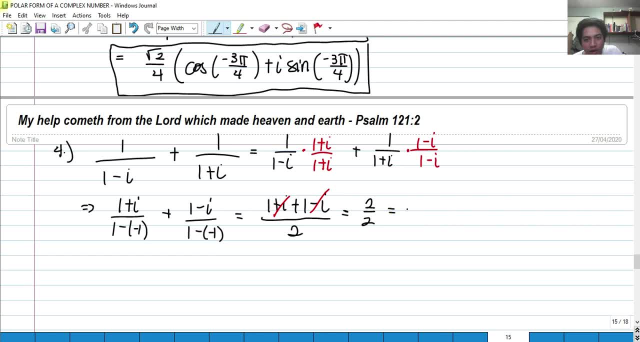 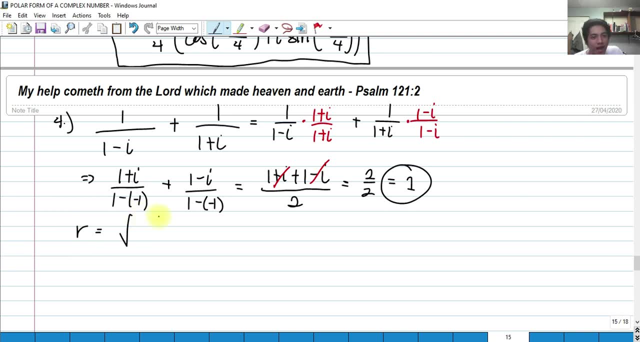 have 1 plus 1 is 2 over 2, or in other words, we have 1. we simplify it as 1, okay, and get the polar form of that. so we have 1 squared plus 0 squared, okay, and that is equal to 1. our theta would be: 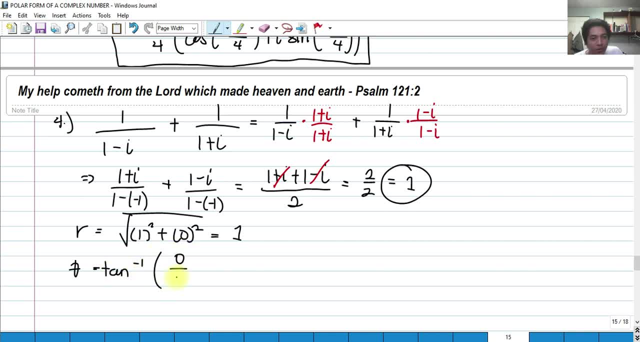 arc tan of y, which is 0, over 1, which is actually calculator, will give us 0 value. okay, or, upon inspection, that would give us 0 value. this 0 is correct, okay, because in the diagram that one is located here. so this is the positive x-axis from which we reference. 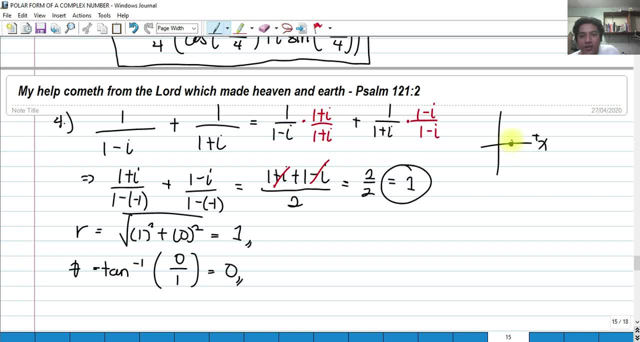 or we refer our theta, so it does not have any angle. so it's actually correct that this is 0. okay, so our answer in getting the polar form of that, okay, therefore, that should be r cosine theta- r cosine theta, which is 0, plus i sine theta, which is 0. so or in other words, okay this if we simplify. 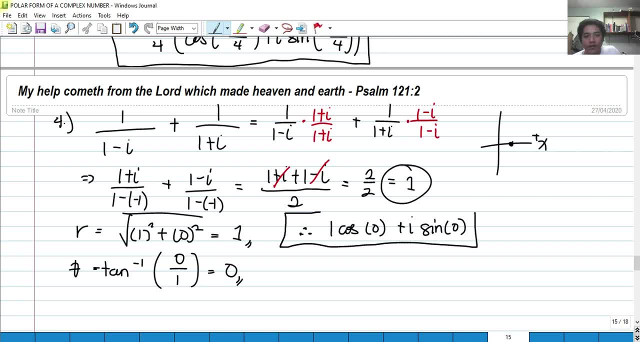 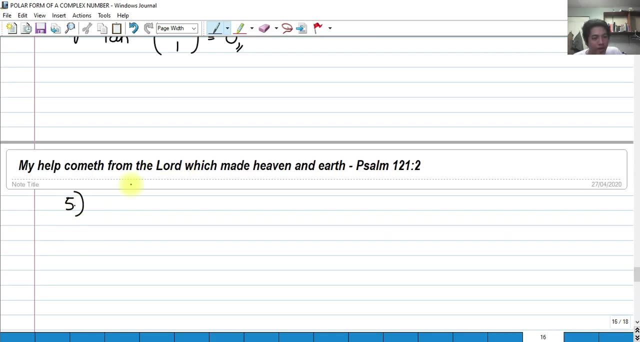 this: this is simply equal to 1. okay, sine 0 is 0, cosine of 0 is 1, which is simply equal to our value of 1. so for number 5, let's try to solve some problem. number 5: we have 2 minus i over i. 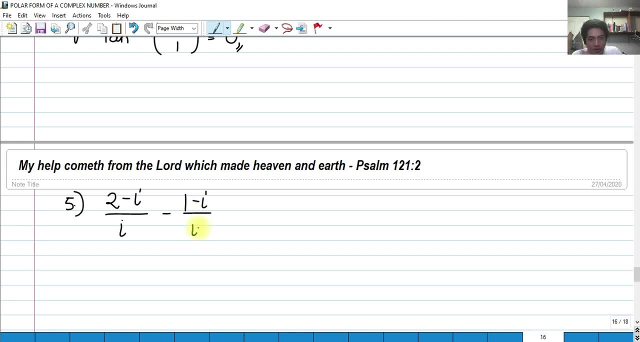 minus 1 minus i over i. as you can see, they have the same denominator, so we can actually rewrite this as 2 minus i. we distribute these so we have minus 1 plus i all over i. so, as you can see, we have some cancellations here. negative i. 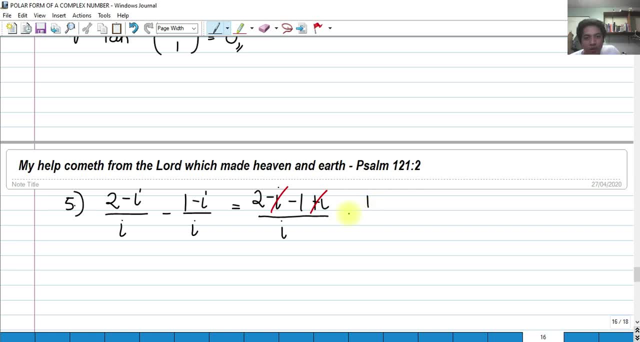 plus i. then we have 2 minus 1, that is, 1 over i. so we need to simplify this. okay, we need first to simplify this by multiplying it by the conjugate of the denominator negative i. so what will happen here is that we have negative i all over negative i times i is negative, negative i squared, but we 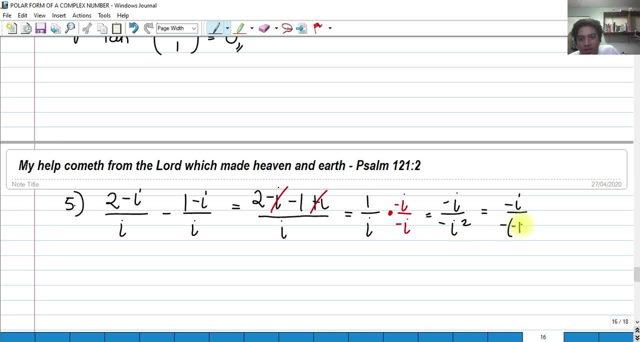 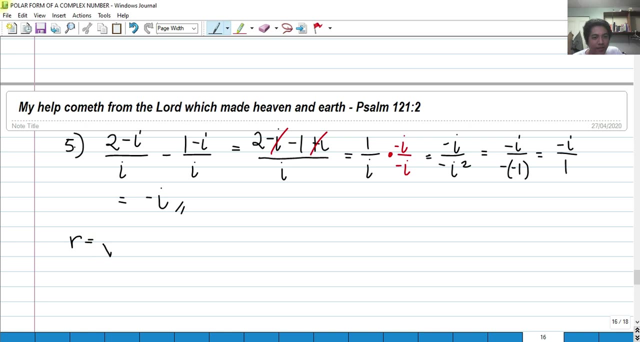 know that i squared is negative 1, so we have negative i all over 1 and that is equivalent to negative i. so our simplified form for the rectangular is simply negative i. so if we get the r and theta of this, this should be 0 squared plus negative 1 squared, which is actually 1. 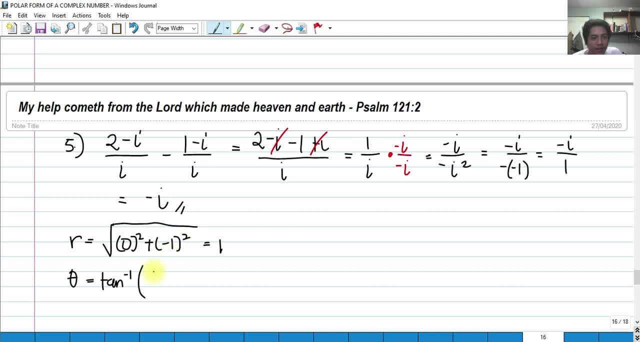 our theta in here is arc tan of negative 1 over 0, which is mat error or undefined mat error if you are using calculator. so by inspection we know that the negative i in the organ diagram is located here. okay, that's the negative i. this is the positive i. so 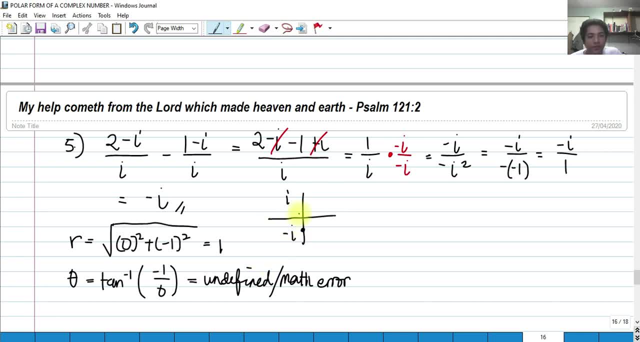 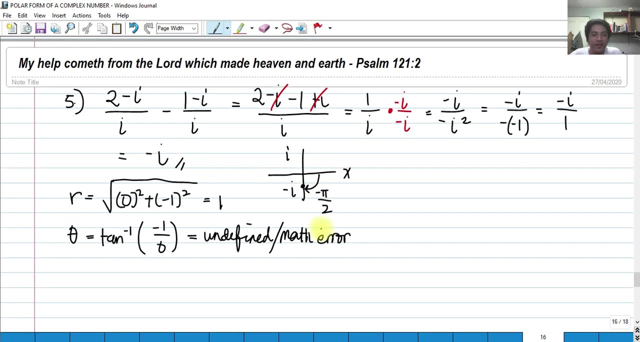 so what would be our angle? okay, if, if we have this, so if we measure this clockwise from the positive x, we have a negative angle, and this angle is negative pi over 2, okay, which is negative 9. so by inspection, we have an angle of negative pi over 2. okay. 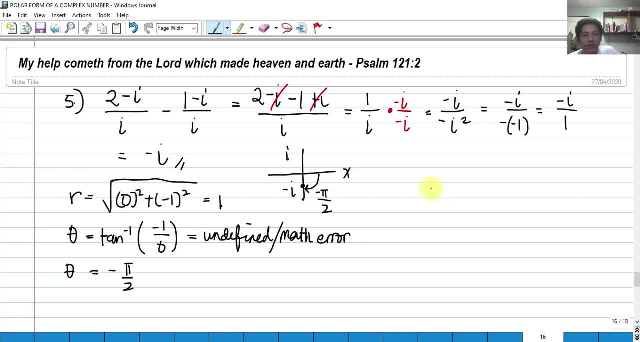 so our uh polar form for this negative i, negative i should be r, okay, or one cosine of negative pi over 2 plus r, which is one, so i'm not gonna write that. so we have i sine of negative pi over 2.. so this is the polar form of our uh. this should be our polar for polar form. so this wave effects. 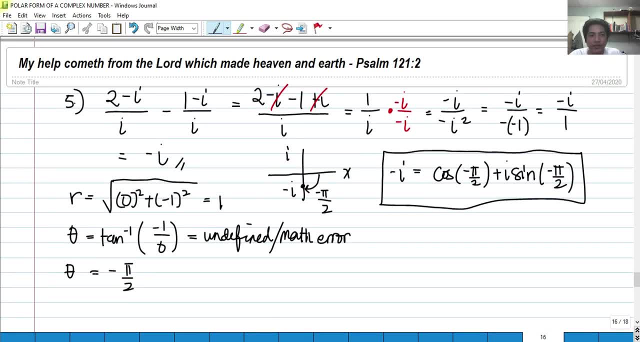 the negative i. so in in circuits it's actually represented as uh, uh, this value. so we have one, i think, angle okay, one angle negative pi over two: okay, in your calculator you can also do that, but for now we are doing it for the complete computation. so number six for number six. 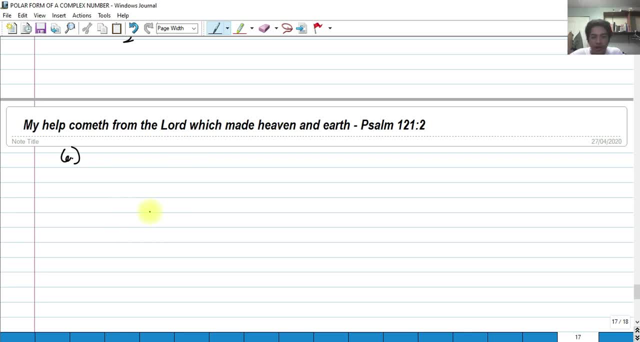 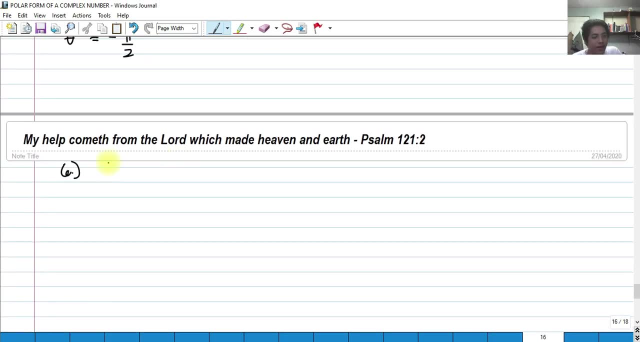 okay, number six. we have. i think it's number six. it's number six. we have a negative four square root of two minus four square root of two. i, it's easy. okay, because it's already simplified. you don't have any denominators, so our r, our r, should be negative four square root of two. 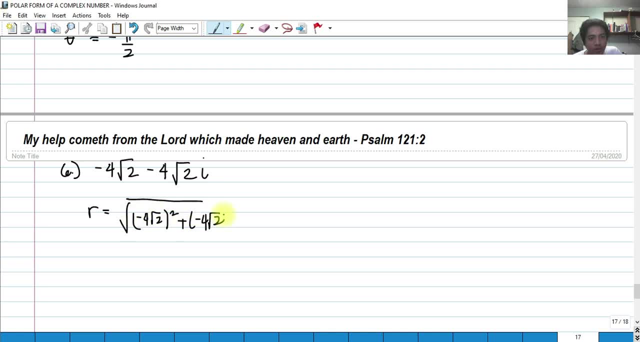 squared plus negative four, square root of two. we have squared, so the value of r should be eight. our theta should be arc tan of simply one, because it's it's really the same. okay, so we have arc tan of one, so our calculator will give us pi over four. we know that this is located in the quadrant three. 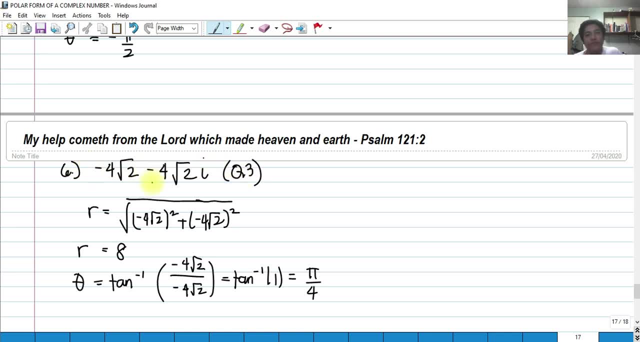 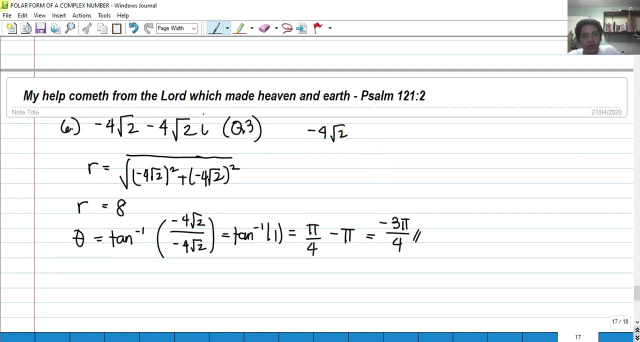 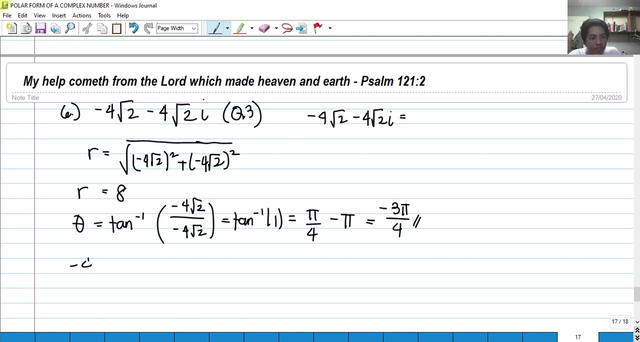 third quadrant because it is negative and negative. so we need to subtract pi from it to get the correct angle. so we have negative three pi over four. so therefore, our answer for getting the uh polar of this polar coordinates or polar form- let me just rewrite this here, it's much spacious. so we have: 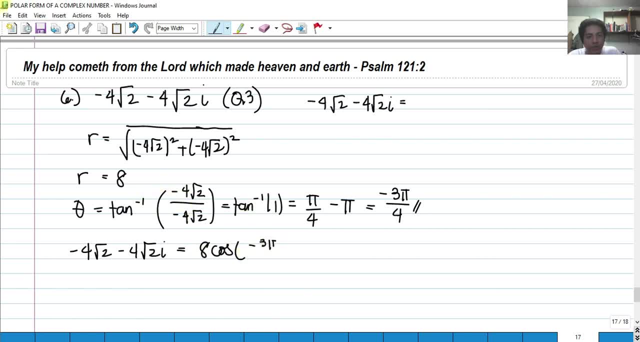 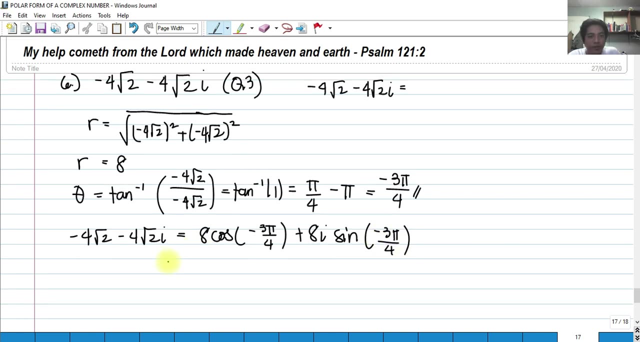 eight cosine of negative three pi over four, plus we have uh i sine, or sorry, we have eight i eight i sine of negative three pi over four. we can factor out eight, so we have eight cosine of negative three pi over four, plus i sine of negative three pi over four. so that is our. 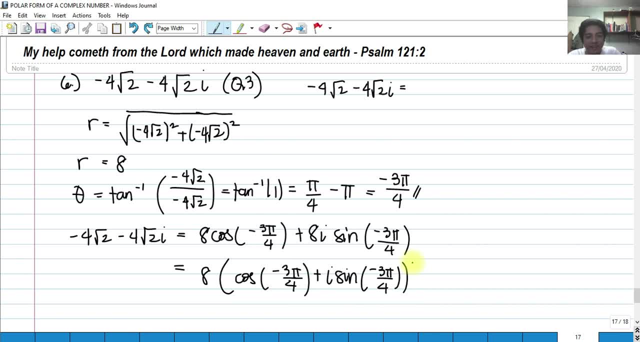 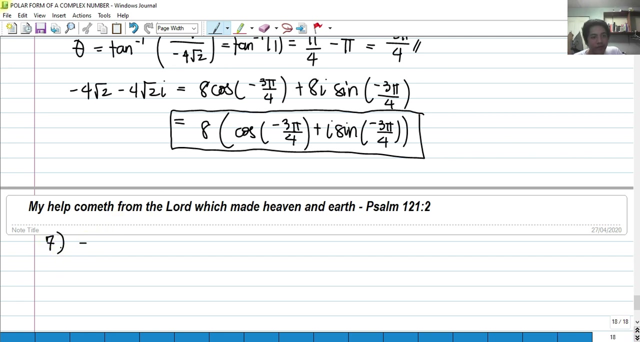 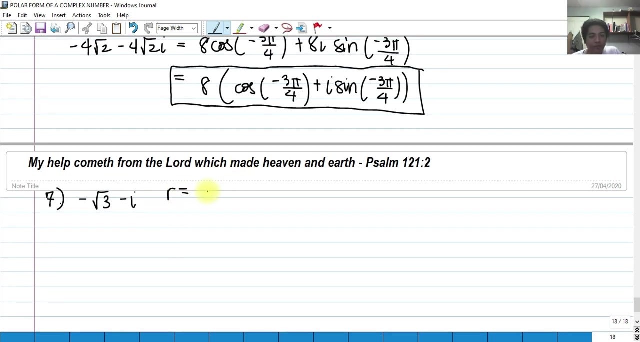 answer: oops. so this should be our answer for this problem. number six: okay, so let's now proceed to number seven. for number seven, we have negative square root of three minus i. it's this pretty straightforward, so we can apply the formula. so: negative square root of three. 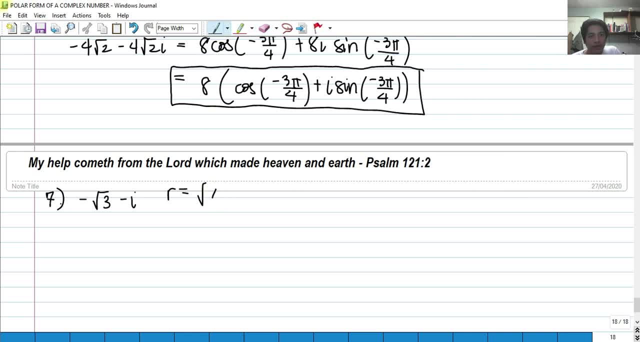 oops, we have negative square root of three squared plus negative one squared. so if we evaluate this, this should be two ive ç. you must plot onto the square root of three hyperbolic square root over three, square root of three pi k, which will give us a sign that we'reян. 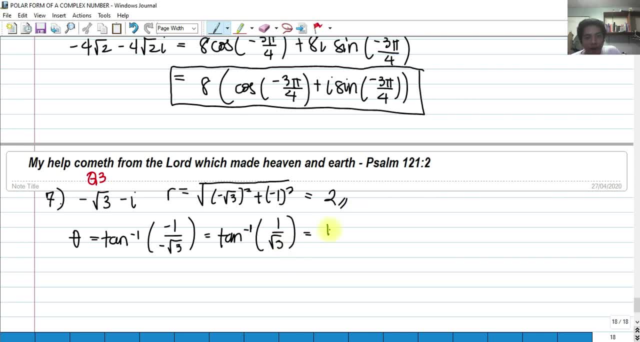 okay, because we'll have to now calculatenine two to the same number, times four, pi over 6, so we need to again subtract pi. okay, because we are using calculator, subtract pi from it, okay, and to get the real, okay, uh, angle or argument. so our answer: 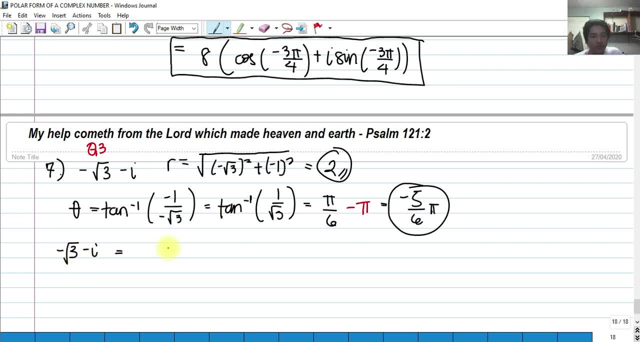 in getting. the polar form of this should be r cosine of theta, that's 5 pi negative 5 pi over 6 plus 2i sine theta, negative 5 pi over 6, or we can factor out 2, so we have cosine of negative 5 pi. 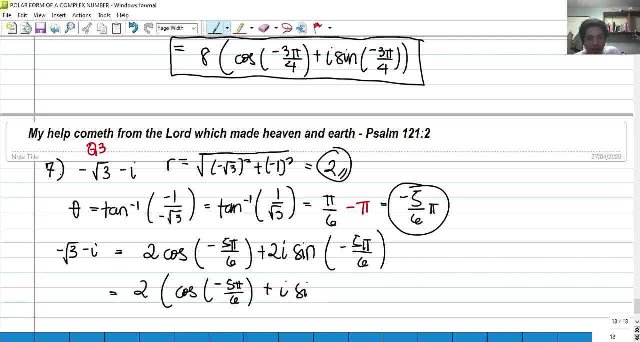 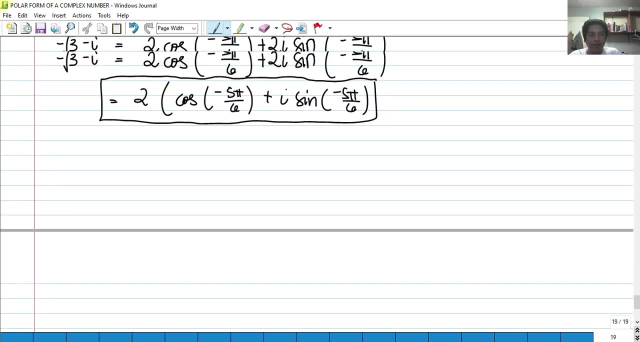 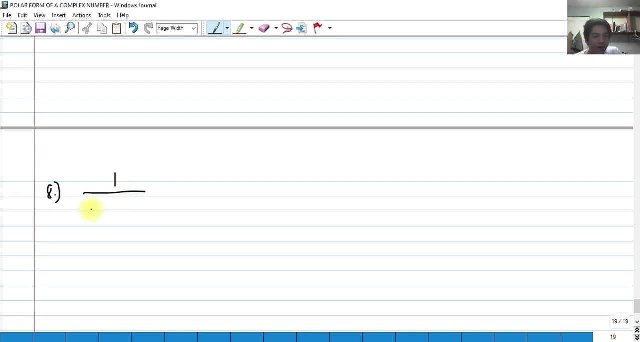 over 6 plus i, sine of negative 5, pi over 5, 6. so this should be our answer for this problem. so let's go now to our last problem. right, maybe for problem number eight. so get or transform this into polar form, this complex number. so we need to simplify this, first by multiplying it by its conjugate. 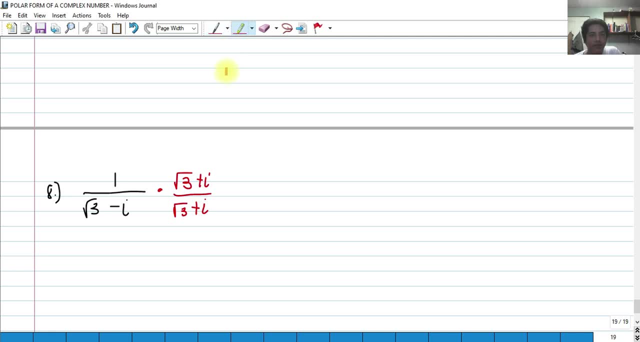 square root of 3 plus i. so we. what will happen is this: would be square root of 3 plus i, square root of 3 times square root of 3, that's 3 negative times positive. that's minus. we have negative i plus i, squared. 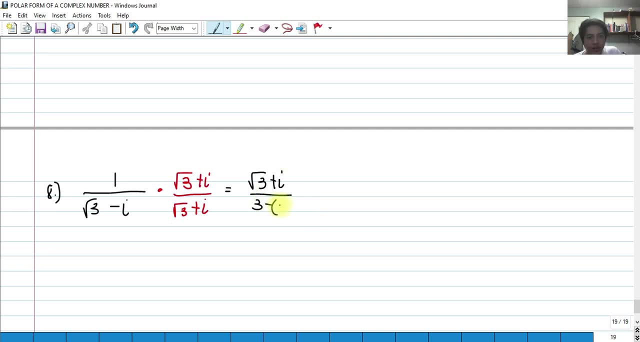 multiplied by i squared, that should be negative 1, i squared is negative 1. okay, so we have square root of 3 plus i all over 3 plus 1, that's 4. so let me just rewrite this square root of plus i all over 4. so in other words, that is square root of 3 over 4 plus one-fourth of i. 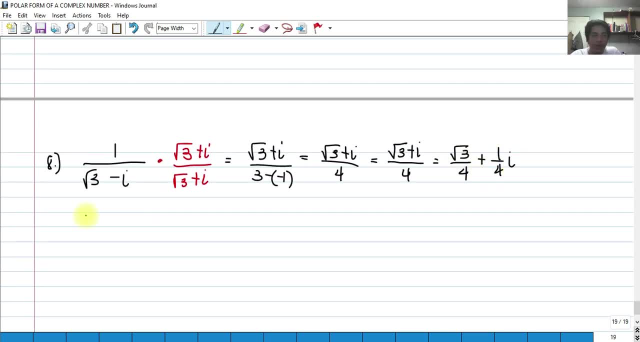 so it's pretty straight forward here that we can get readily the r and the theta. so we have, for the r, that's square root, of 3 over 4 squared plus one-fourth squared. take the square root of that so it turns out to be one-half, and theta for arctan that's y over x, one-fourth over square root. 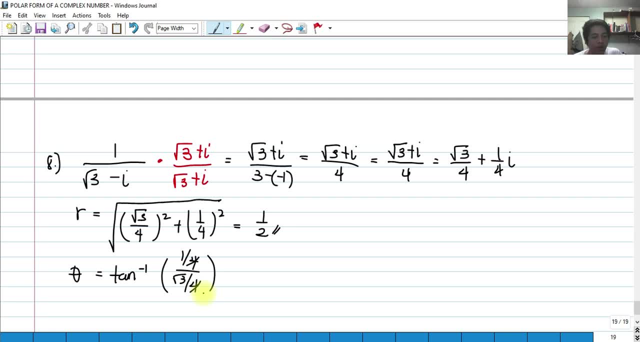 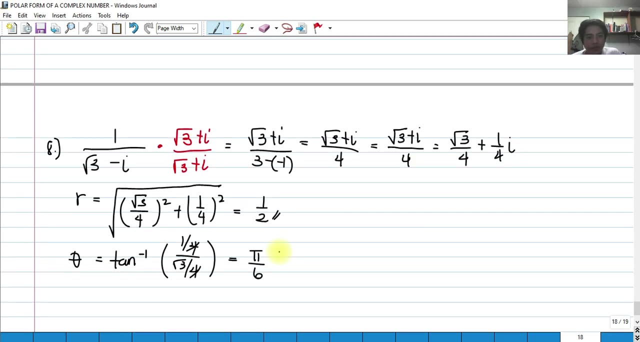 of 3 over 4. these two will cancel our calculator, will give us pi over 6. but take note again, okay, take note- that in this problem we need to subtract or add pi over 6, because the given complex number is given or or located in quadrant.